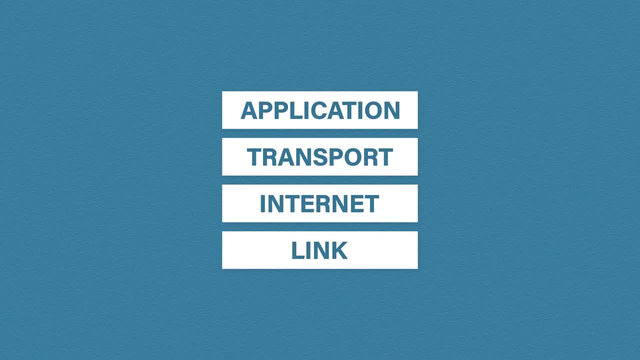 Here is the TCP IP model: Four simple layers- application, transport, internet and link. And just like the OSI model, it's numbered from the bottom up, but the direction depends on if you're sending or receiving traffic. So this is the original model, but it has been updated. Here is the brand new, freshly designed model. One extra layer and one renamed layer. That's it. The link layer has been split into data link and physical, and the internet layer has been renamed. the network layer. Simple, right. It gets even better when we compare the TCP IP model. 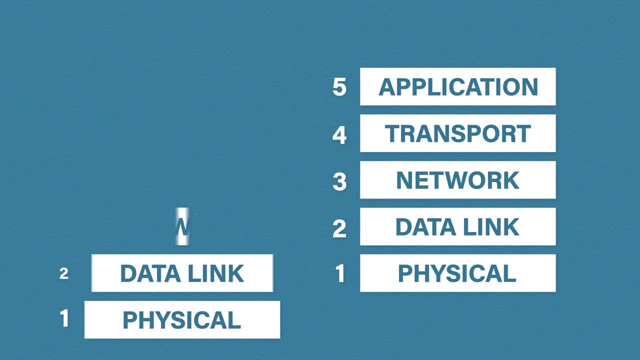 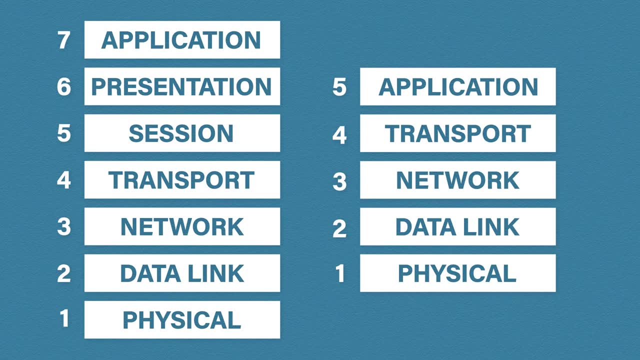 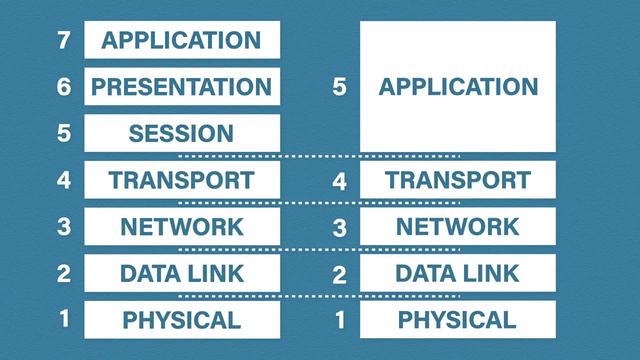 to the OSI model. Now, if you remember, the OSI model has seven layers compared to our five here. But when you look at it you'll notice the application presentation and session layers are just shown as application layer in the TCP IP model. All the other layers line up nicely. 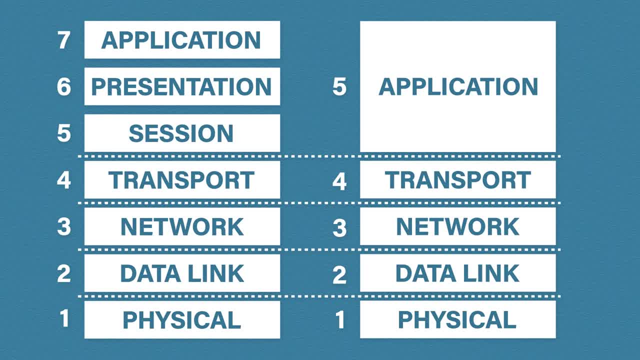 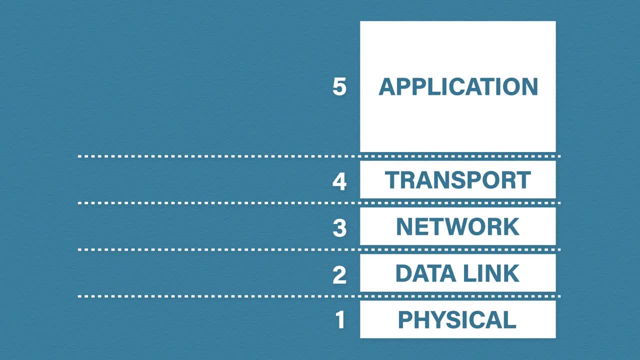 which is great, because we should already know the concept of how this works. So let's remind ourselves about the protocols and devices at each layer. At the application layer, we have application protocols such as HTTP, FTP and SMTP, The two most common transport. 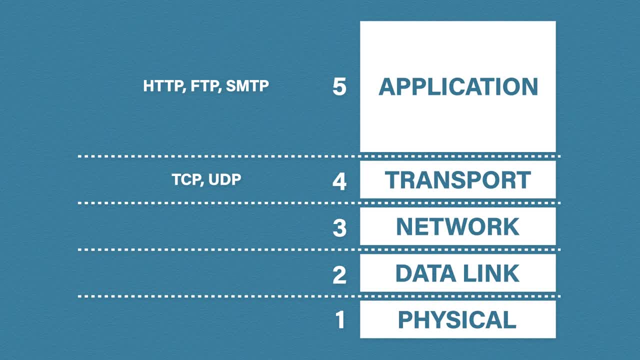 protocols are TCP and UDP. Port numbers are also added here. At the network layer we have the internet protocol or IP. Routers also operate at this layer. The data link layer contains ethernet switches typically operate at this layer, although you can get layer 3 switches that have some. 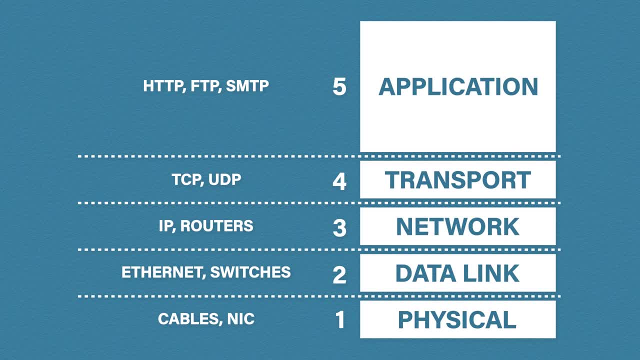 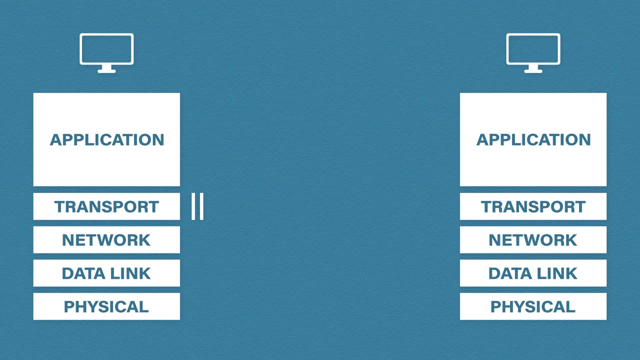 routing capabilities. Finally, we have the physical layer. Think of everything we can touch and feel here, Things like cables and network interface cards. Okay, so, as we send data, each layer will add its own bit of information. This process is called encapsulation. When we hit the physical layer, the 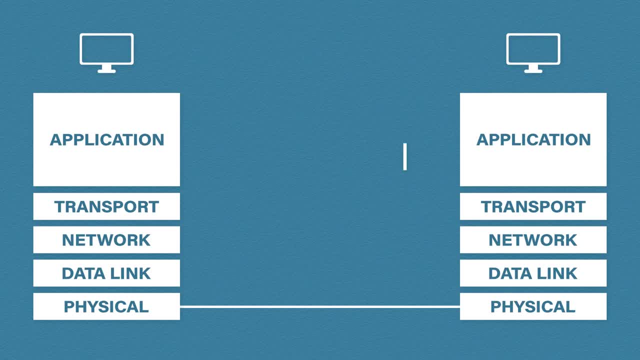 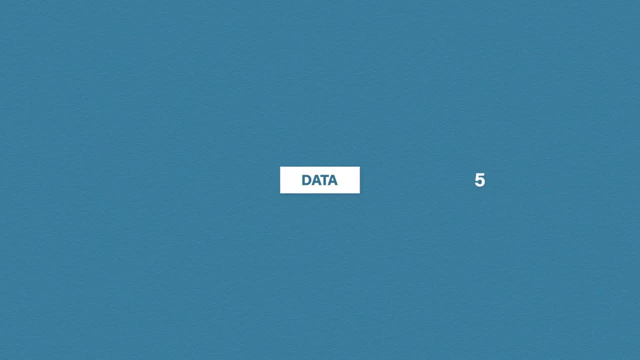 data is then sent to the receiving device. The receiving device then starts to decapsulate the data. We saw this in the OSI model, but in this video we're going to take a closer look. We start with our application data at layer 5.. This is then passed down to the next layer, where 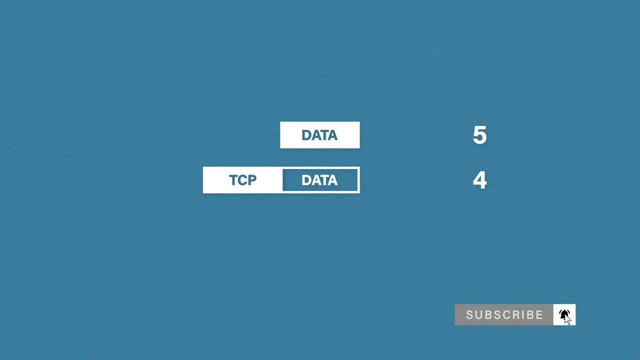 the transport information is added. Let's say it's a TCP header. Each time a header is added, this will contain specific information. For example, a TCP header will contain things like the source and destination data, Port number, sequence numbers and a few more bits of information. We'll go over this in more detail.